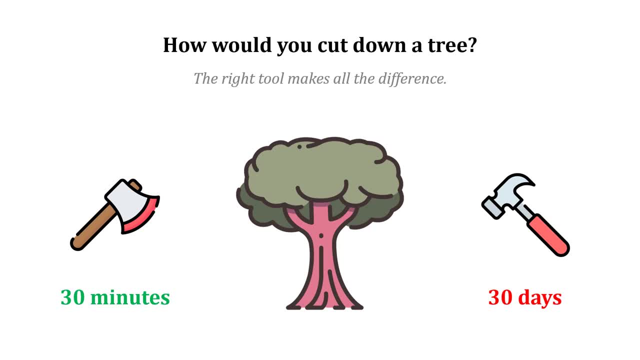 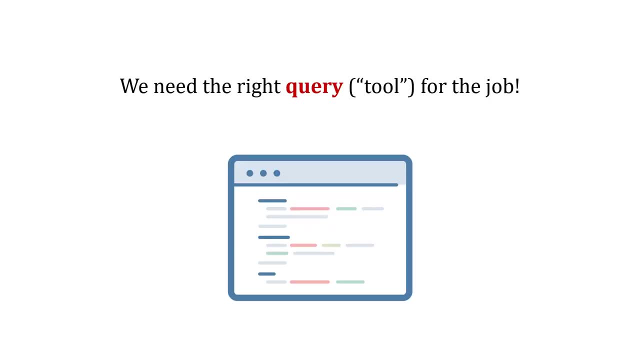 it could take literally 30 days of us just banging on that tree. In this scenario, the tool makes all the difference. It's the same thing with our SQL queries: We need the right query or tool for the job We're looking for- efficiency. Now let me talk about a few optimization tips that might be. 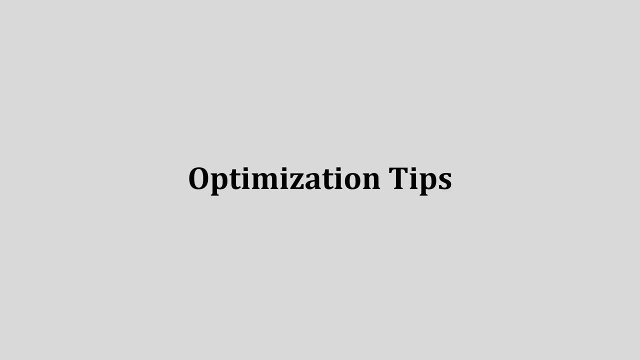 helpful as you work to make your queries more efficient, And so I'll walk through these at a summary level And I'll go through them one by one, And I'll talk about how to optimize your query results. So let's go through them in more detail in just a minute, So select only the 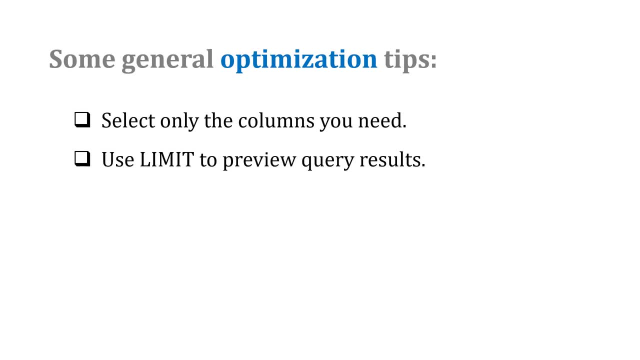 columns you need. That's the first tip. Use limit to preview your query results. Use wildcards only at the end of a phrase. Avoid. select distinct if you can, And then run large queries during off peak hours. Let me explain each of these in a little bit more detail And I'll show you an. 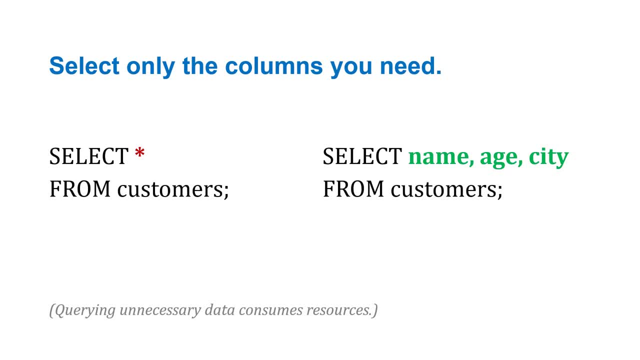 example too. So select only the columns you need. If we're querying unnecessary data, that's going to consume more time, So let's go through them in more detail And I'll show you an example too. So in this example, maybe instead of using select star, go with select name, age and city. 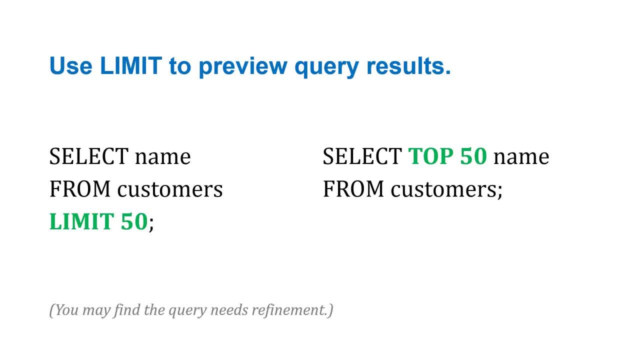 if that's all that we really need, Then use limit to preview your query results. When you first run a query, it might be helpful to just look at a few records to see if the results are what you expected, And you could use limit to do that And, depending on your database, it may be limit or top. 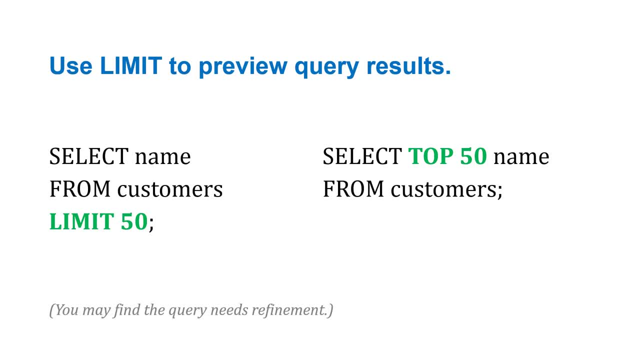 select name from customers limited to 50 results or select top 50 customers limited to 50 results. So it could be limit or top And then use wildcards only at the end of a phrase. So if you have wildcards in your where clause, what you'd like to do is to kind of keep that at the end. 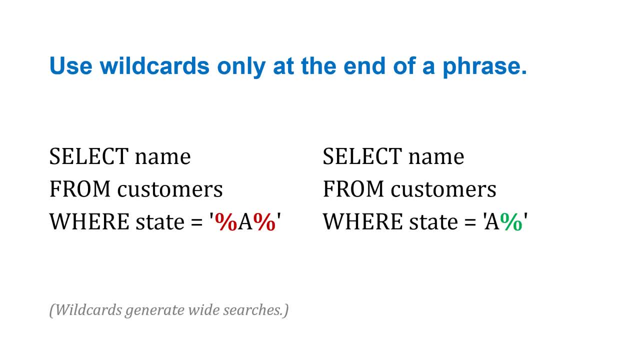 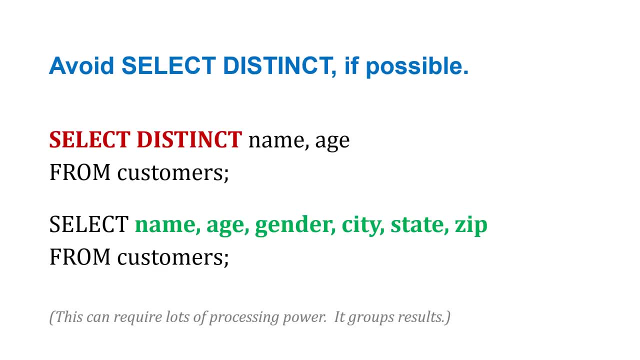 which is on the right, because wildcards generate wide searches And it's really the widest search possible. if you've got those wildcards at the beginning and the end of a phrase, Then avoid select distinct if you can, Without going into too much detail. this requires lots of processing. 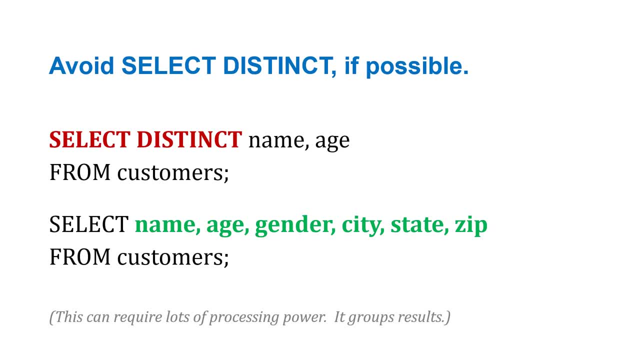 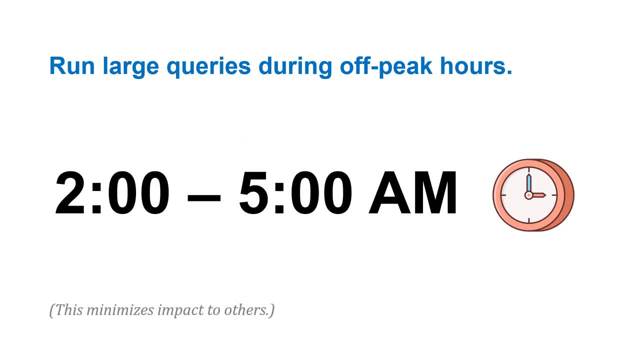 power. So it's really important to keep that in mind And then use limit to preview your query results. So, instead of using select distinct, you might just select enough fields to give you the unique results that you're looking for And then finally run large queries during off peak hours to minimize